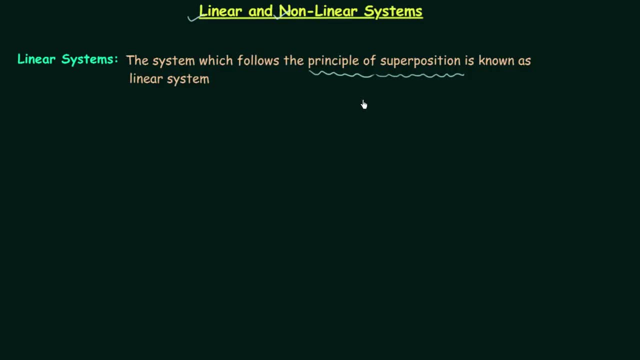 the principle of superposition. So the important thing is to understand what is the principle of superposition. This principle of superposition, or the law of superposition, is sufficient, and sufficient condition to prove the linearity of the system. So if you can prove the system, 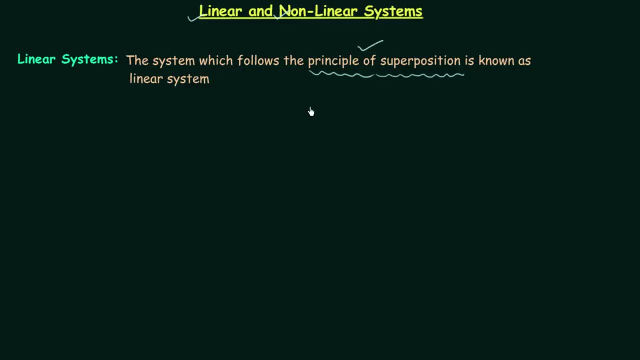 is following the principle of superposition. it is definitely going to be linear system because this particular principle is the necessary and sufficient condition. So let's first understand what is this principle of superposition? The principle of superposition is combination of two different laws. The first law is known as law of addition and 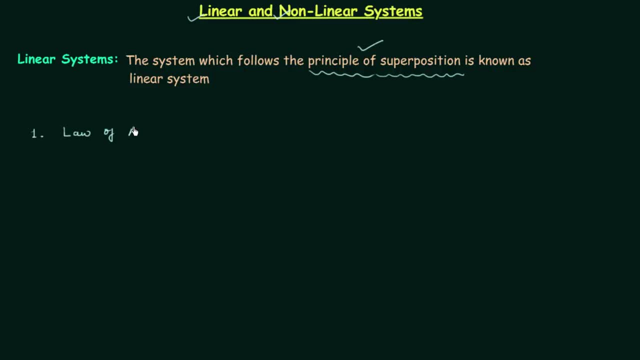 the second law is known as law of homogeneity. So we will first understand the law of additivity and once we are done with law of additivity, we will understand law of homogeneity, and the two laws combined will form the law of superposition. So let's see what do we mean. 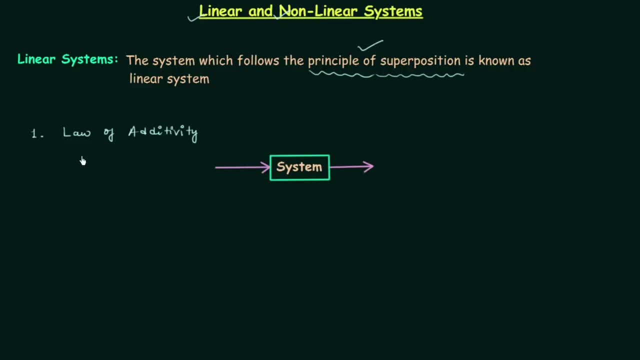 by the law of additivity, the output y2t. So this is what we have, and now we will add the two outputs y1t and y2t. we will add: 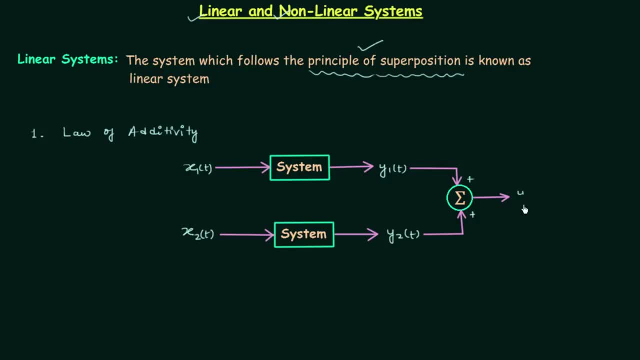 After adding y1t and y2t, we have y1t plus y2t. So this is what we will do in first step. In second step, instead of adding the outputs y1t and y2t, we will add the two inputs x1t. 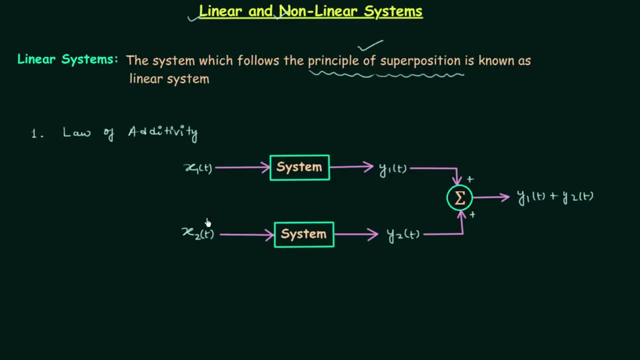 and x2t and the result of addition. x1t plus x2t will act as the input to the same system and the output generated we will compare with this result. So let's perform the addition of the two inputs first. After adding the two inputs, we will have x1t plus x2t, and x1t plus x2t is now acting as: 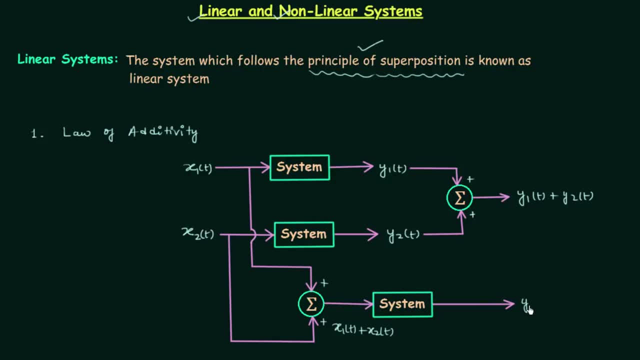 the input to the same system And let's say the output generated is y2t. Now there are two possibilities. The first possibility is that the output y-t is same as y1t plus y2t, and the second possibility is that the output y-t is not same as y1t plus y2t. 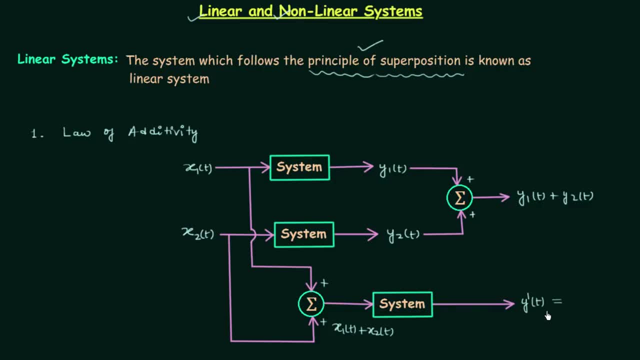 So I will write down the two possibilities. y-t is same as y1t plus y2t. This is the first possibility And the second possibility. The second possibility is that it is not same as y1t plus y2t. 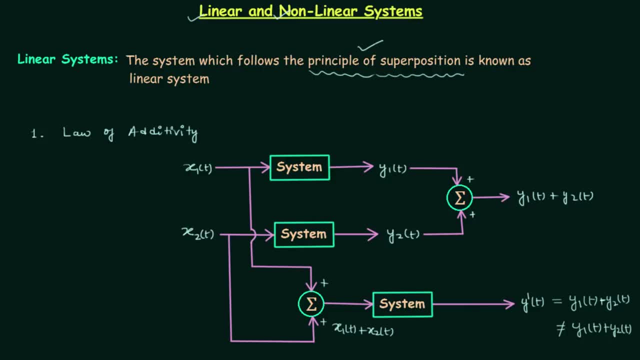 Now, in the first possibility, when the two results are same, we say the system is following the law of additivity. It is following the law of additivity. And in the second case, when the two results are not same, it is not following the law of. 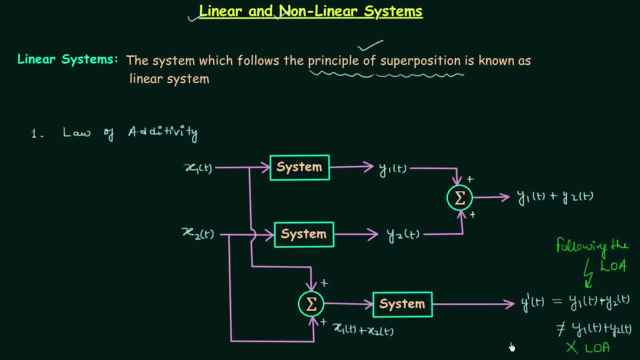 additivity. So I think you now understand what do we mean by law of additivity. You have to give two different inputs to the system and you have to record the two outputs. Then you need to add the two outputs and you need to record the final result. 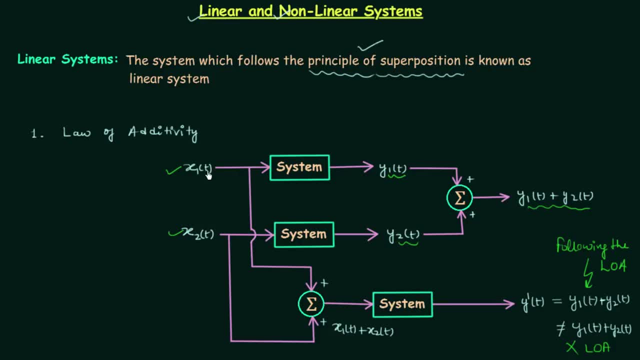 After this, instead of adding the two outputs, we will add the two inputs directly. As you can see here we have added x1t and x2t, and then we will feed x1t plus x2t to the same system. So the system is not changing throughout these operations. 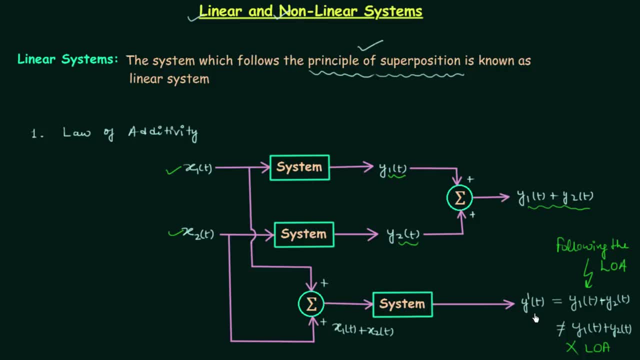 We have the same system and in the second case, let's say the output is y-t. Now compare the two results. If they are same, then the system is following the law of additivity And we can move on to check the law of homogeneity, because the principle of superposition is. 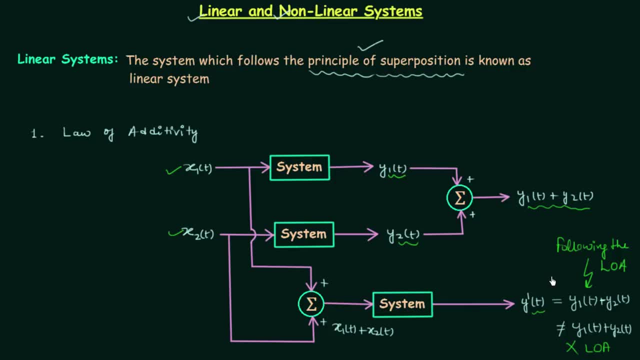 composed of law of additivity and the law of homogeneity, And if any one of these two laws are violated, then the principle of superposition is not same. The principle of superposition is violated and the system is non-linear. So when you check the law of additivity and you find the two results are not same, then 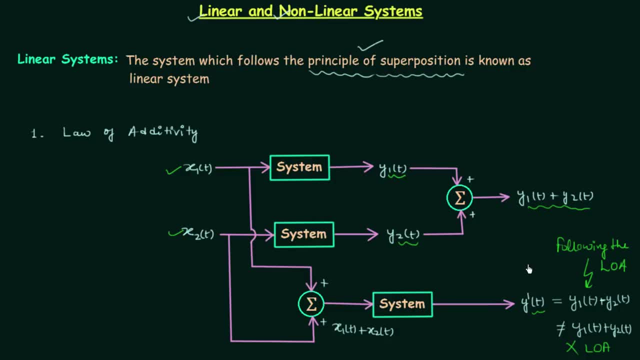 stop right over there and you can write down. the system is non-linear. There is no need to check for the law of homogeneity, because the law of additivity is violated and thus the principle of superposition is also violated, and the system is non-linear. 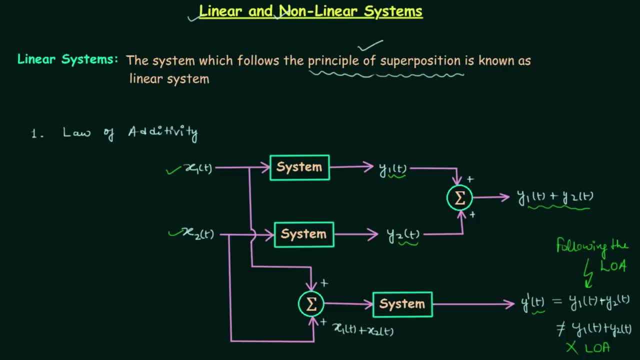 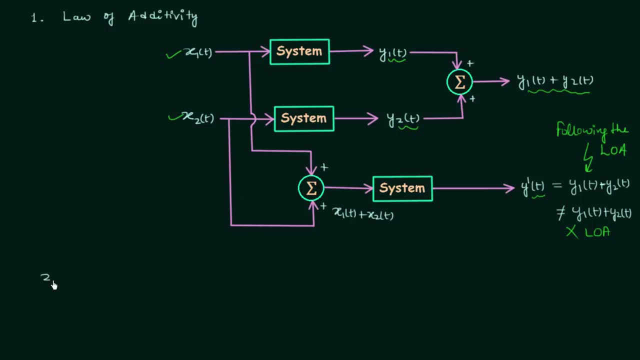 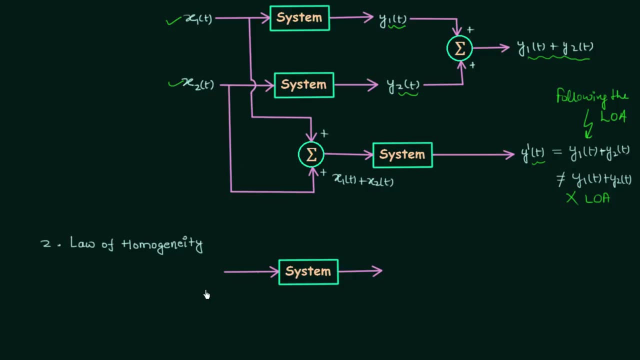 Now we will discuss what do we mean by law of homogeneity? The law of homogeneity is a very simple law to understand. It is very much similar to the law of additivity and as we are checking the linearity property of the given system, we cannot change the system while checking if the system follows the law. 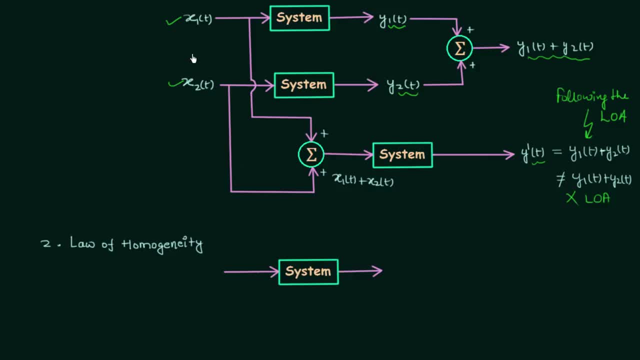 of homogeneity or not, The system will remain same as it was in case of law of additivity. So we are having the same system and let's say the input this time is xt and the output generated is yt. Now this time, Let's say: 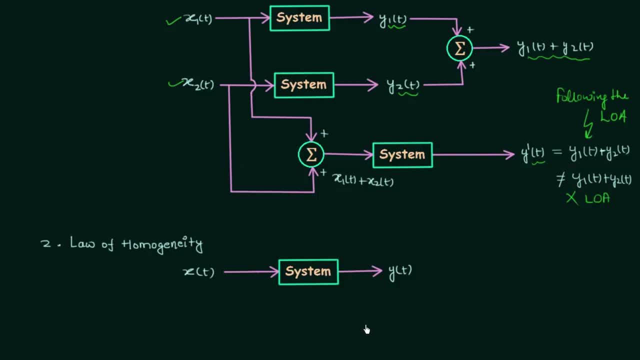 We will not perform any addition, but we will perform the multiplication. We will multiply a constant k to the obtained output yt. After multiplying k to the output yt, we will have k times yt. So this is all we need to do in step number 1.. 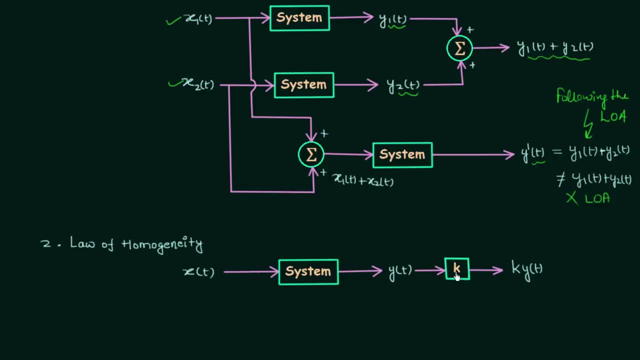 In step number 2 we will multiply the same constant, the same constant k, to the input xt, and the obtained result will act as the input to this system, And then the generated output we will compare with kyt. That's why I was telling you law of homogeneity is very much similar to the law of additivity. 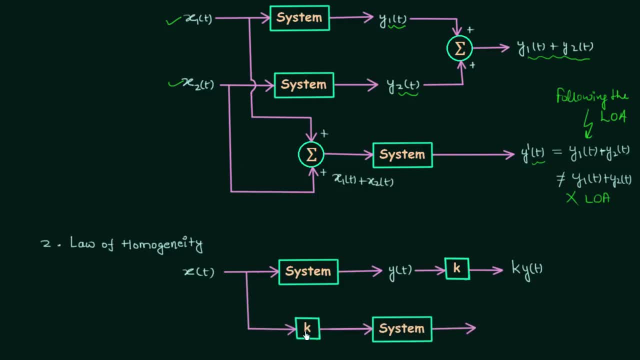 So let's complete our step number 2.. After multiplying k to xt, we will have kxt, and this kxt is the input to this system and the output generated is, let's say, y-t. Now again, there are two possibilities: y-t minus k. 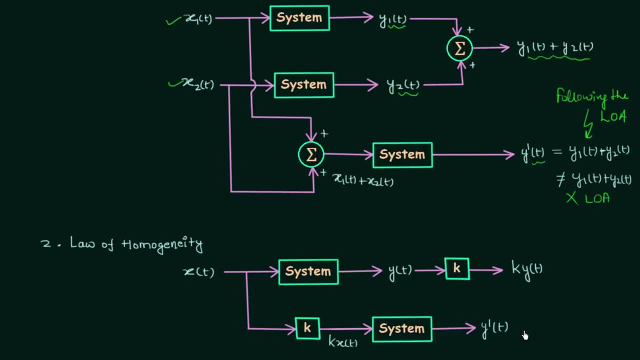 y-t may be equal to kyt or it may not be equal to kyt. So in first possibility, y-t is equal to kyt and in second possibility it is not equal to kyt. Now, when y-t is equal to kyt- the first possibility- we say- the system is following the law of 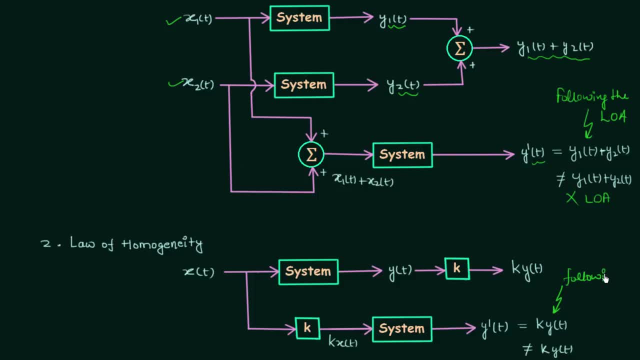 homogeneity, The system is following the law of homogeneity And in case number 2, or the possibility number 2, when y-t is not same as kyt, we say the system is not following the law of homogeneity. So this is all you should know about the law of homogeneity and there is no compulsion on. 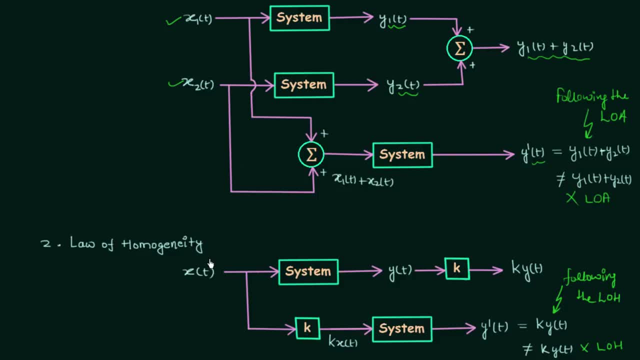 checking the law of additivity first. You can check the law of homogeneity first, and when you check the law of homogeneity first and you find the system is not following the law of homogeneity, there is no need to check the law of additivity. 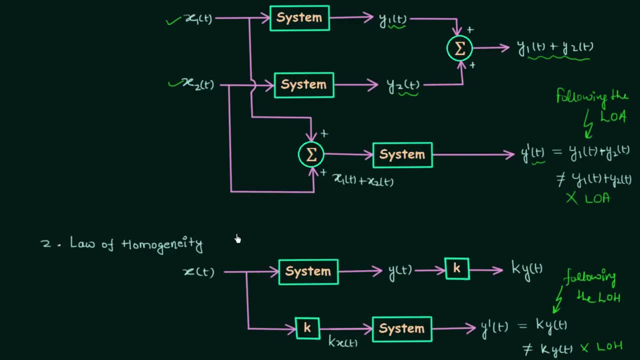 Because the system is going to be non-linear as it has already violated the law of superposition. So I hope you now understand what do we mean by law of superposition. It is combination of two different laws. The first law is law of additivity and the second law is the law of 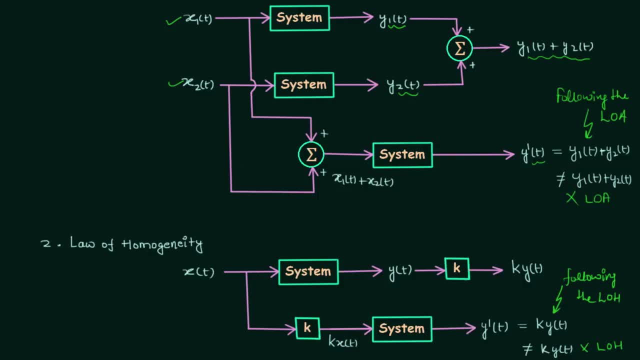 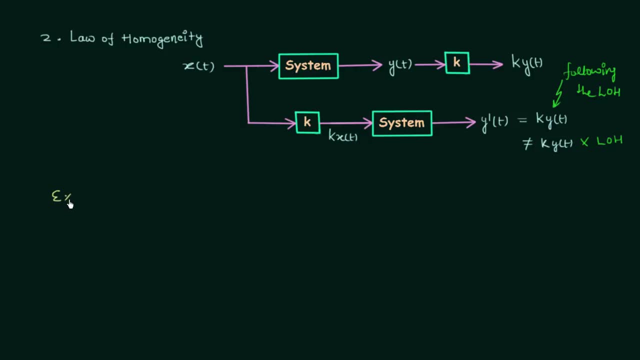 homogeneity. Now we will solve one example very quickly to understand what we have discussed till now. In this example, output yt is equal to x sine t. We need to find out if the system is linear or it is non-linear. For this we will first check the law of additivity and, in order 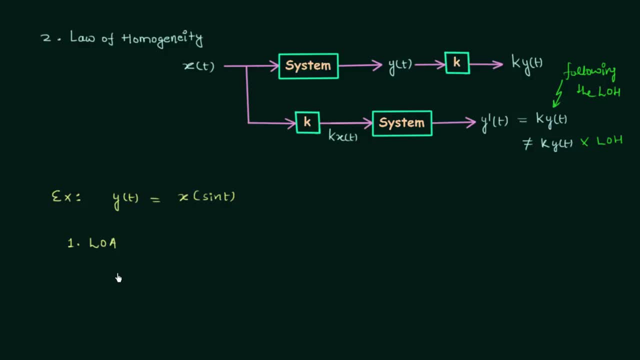 to check the law of additivity. what we do? We add two different outputs generated by the system. when we feed two different inputs, Let's say the first output is y1t and from this relationship we can say y1t is equal to x1. 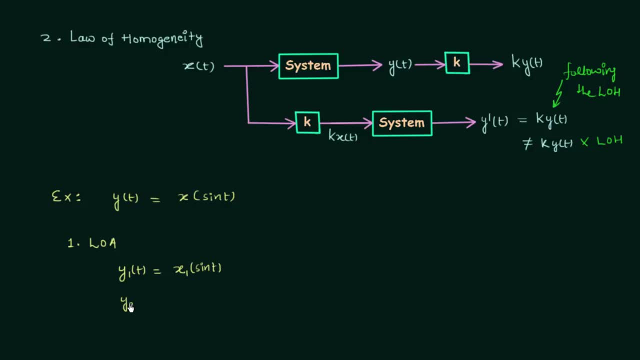 sine t. In the same way, we will have y2t and it is equal to x2 sine t. Now we will add the two outputs, y1t and y2t, y1t plus y2t and it is equal to x1 sine t. 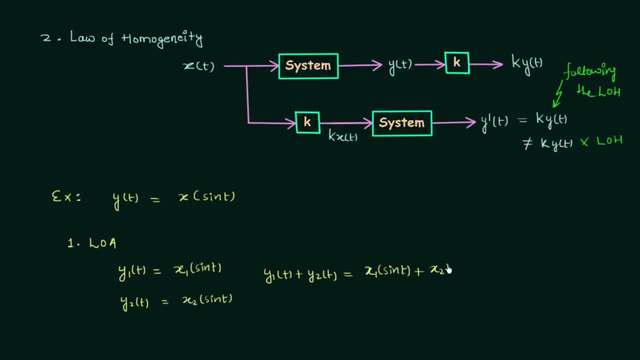 So this is what we have in step number one in order to check the law of additivity. Now, in step number two, instead of adding the two outputs y1t and y2t, we will add the two inputs x1t and x2t. 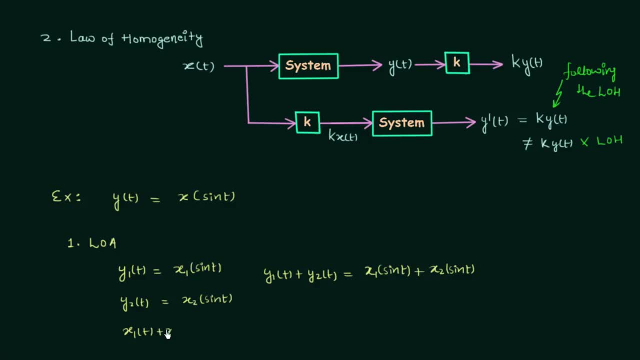 x1t plus x2t and then we will feed it to our system And if you see the property or the functionality of the system, you will find the t in the input is replaced by sine t. xt is the input of the system and the output of yt is equal to x sine t. If you 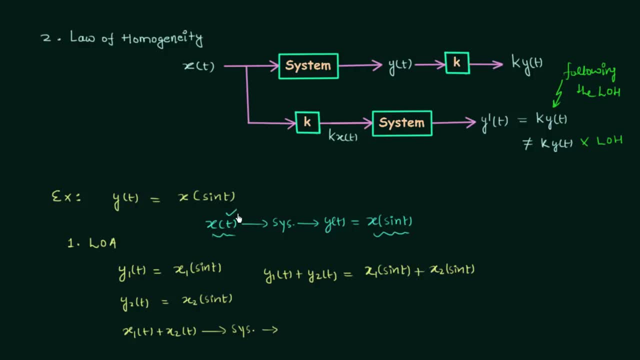 compare xt and x sine t, you will find in place of t we have sine t. So this is the functionality of the system. So in step number two we have x1t plus x2t- Ok, x2t. So in place of t we will have sine t. So let's quickly write down the output of: 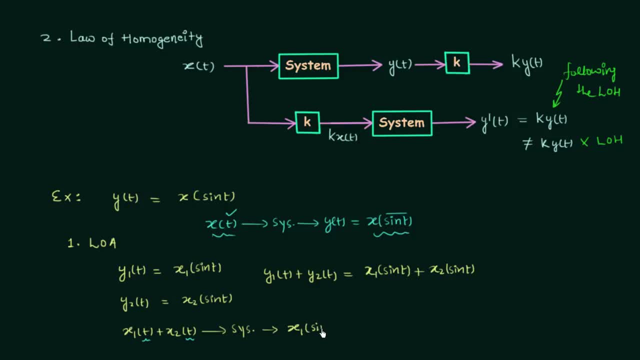 the system it will be x1 sine t plus x2 sine t. And if you compare the two results, if you compare this result here and this result here, you will find they are same. they are same, So we can say that the system follows the law of additivity. Now we will check the 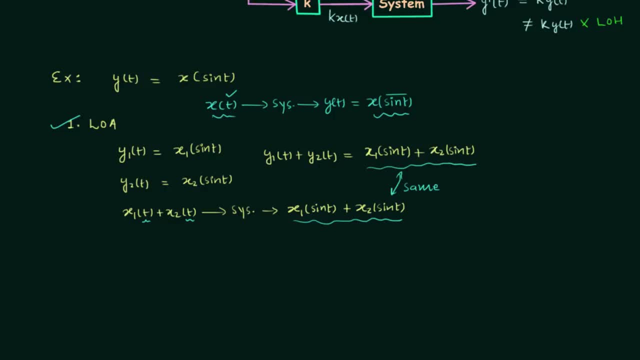 law of homogeneity. In order to check the law of homogeneity, we will multiply constant k to the output of the system. law of homogeneity: yt is the output and it is equal to x sine t. we will multiply k, one constant, to the output. So this side we will have k and this. 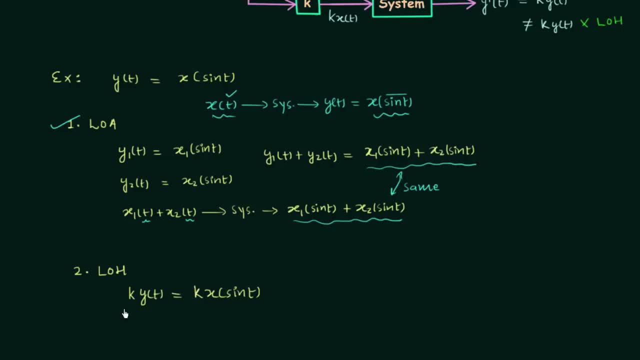 side, we will have x sine t. Now in step number two, instead of multiplying this k to the output yt, we will multiply it to the input xt and then we will feed it to the system. And we already know the functionality of the system: it replaces t by sine t, So we will 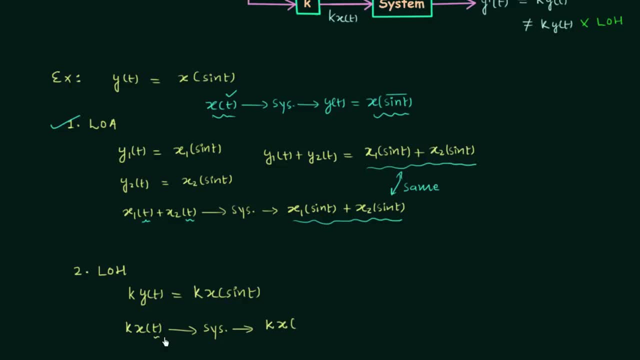 have kx in place of t, we will have sine t. Now compare the two results. you will find they are same. So we can say that the system follows the law of homogeneity. And as the system is following both law of additivity and law of homogeneity, it follows the law of superposition. And as